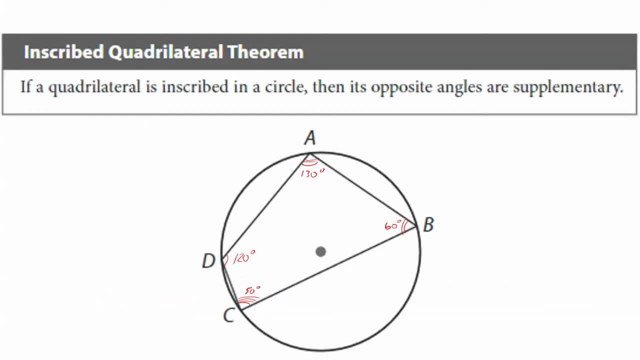 50 degrees. So that's basically what the inscribed quadrilateral theorem is basically saying there. And also, if you remember, a quadrilateral has to have the sum of 360 degrees, And that was from the past, when we had the number of sides. your polygon had minus two times 180 degrees And 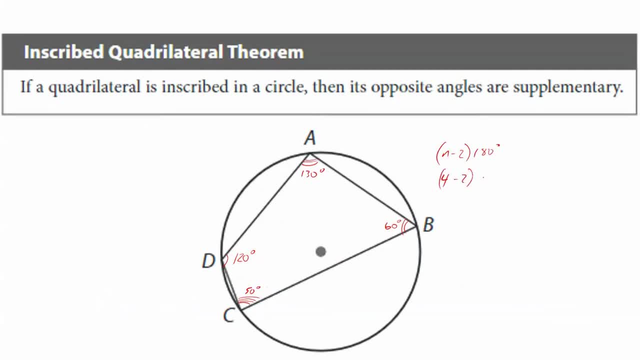 again, a foregone has four sides, So four minus two is two, And two times 180 degrees should equal 360 degrees. So that's just like a little footnote there. All right, so don't forget it's still kind of connected to that concept that we learned. 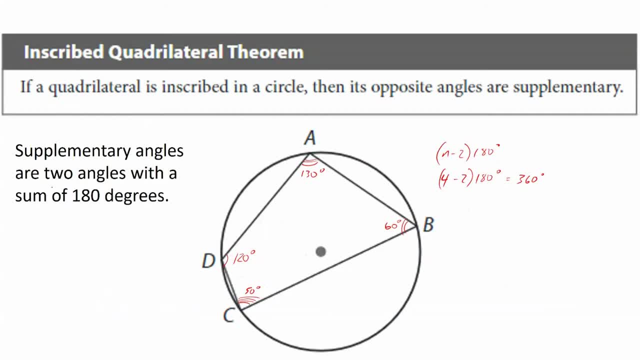 All right. so again, supplementary angles are two angles with a sum of 180 degrees. All right, so that's a very important word there. Remember, inscribed means inside a circle, and quadrilateral quad means four. So just something to note there. 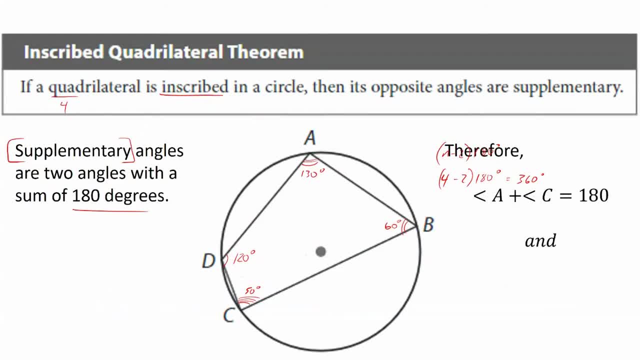 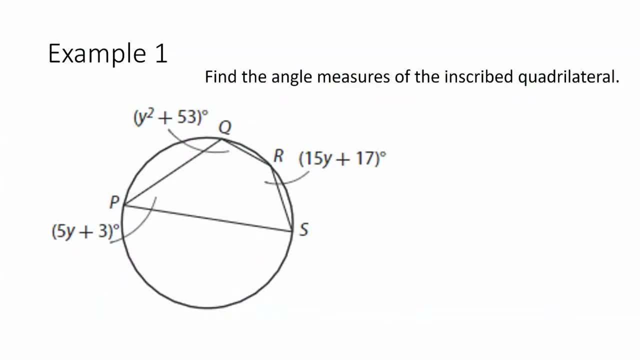 All right. so here's a little bit of this. So, angle A, angle C: right, and that's just an example of how you would write it. okay, for supplementary angles, All right. so example one: find the angle measures of the inscribed quadrilateral. So basically, 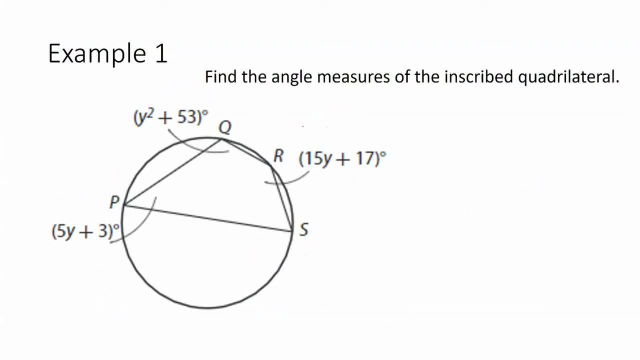 we're just applying geometry, the theorem for inscribed quadrilaterals, and then just using algebra to solve for our angles. So, first things first, we do have some algebraic expressions representing our angles And it looks like our variable is y. Tell me y, All right. so basically, 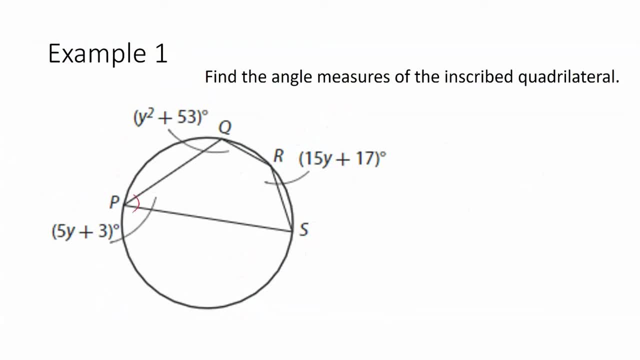 we're going to apply our theorem. So first things first, I notice that angle P and angle R, those are on the opposite side of the square and those are the opposite sides of the square. So sides right opposite angles and they have to be supplementary. that means they have to add up to. 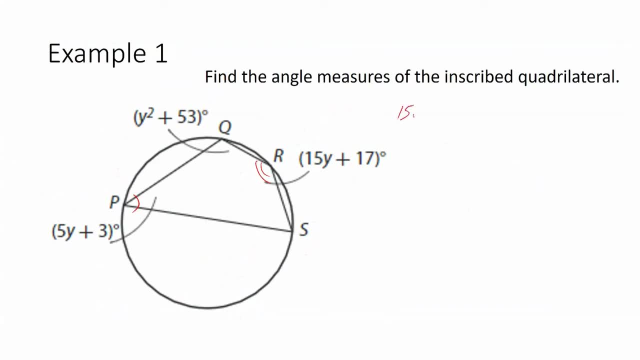 180 degrees. so that means 15 y- tell me y- plus 17. okay, so again, angle r, i'm sorry, angle qrs, all right, plus angle qps have to add up to 180 degrees. so again, that's the general idea. so we have qrs, angle qrs being 15 y plus 17, plus angle qps, which is 5y plus 3, and they all have to. 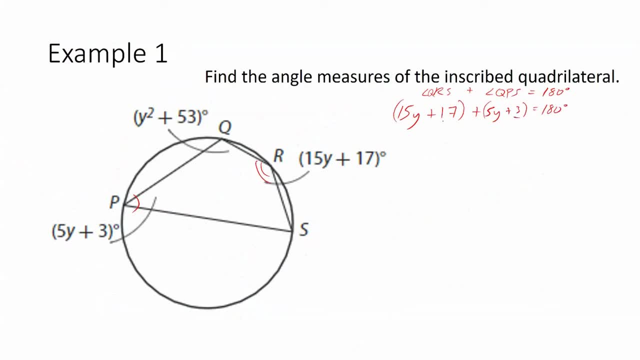 add up to 180 degrees, combine like terms, all right. so we got that 20 there, and then 15 y plus 5 y is 20 y. tell me what? all right, equally, 180 degrees, subtraction property. and don't forget the law of equality, or property of equality. um, what you do to one side, do the other. 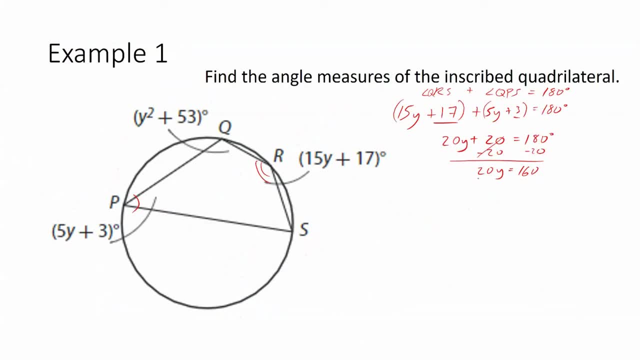 property of equality, and then how to get rid of a multiplying 20 on the left right, because we're isolating the variable, which is y, and then, basically, you should get y equals um eight. so that's not our answer, though. okay, so it's not like algebra, where it's like: oh there it is, there's. you know. y equals this. 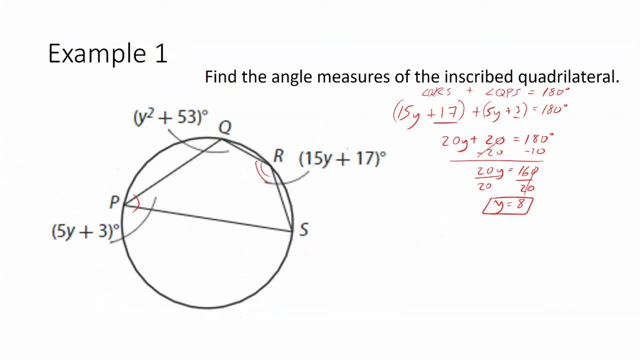 um, no, this is geometry and basically that means we just plug back in our values for y. okay, we can plug it in there, we can plug it in here. so angle r or qrs, should be 15 times 8 plus the 17, so that should. 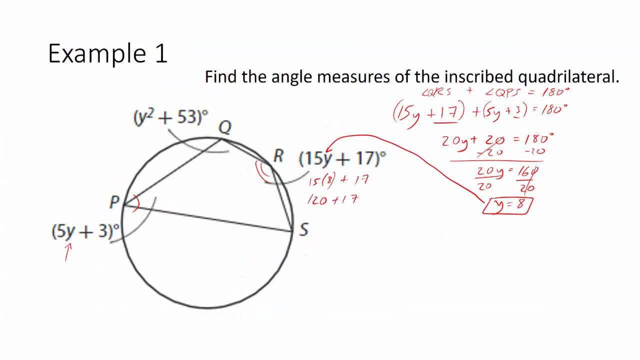 be 120 plus 17, so this angle right here is going to be 137 degrees. now you could plug in uh y here right, 5 times 8 plus 3 and you get 43, or, if you remember, um. basically angle qps and angle qrs have. 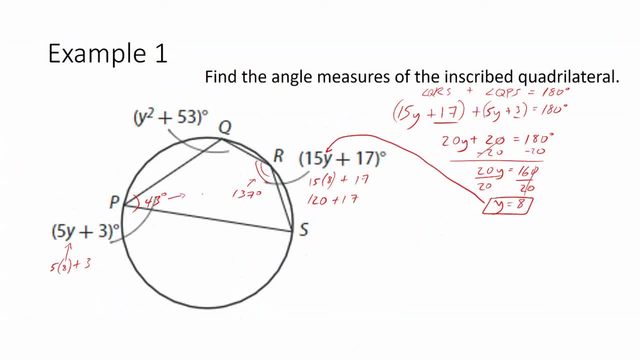 to add up to 180, and you could always just do well, 180 minus 137, and it still gets you the 43 degrees. so that's just something to kind of note there, all right, so let's go ahead and plug in um 8 for. 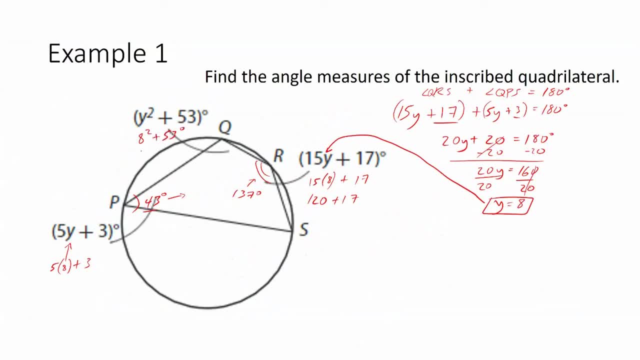 the other angle. all right, that's the 64 plus 53 degrees, and that should give you 117. all right for there. and again, angle pqr and angle psr should add up to 180 degrees. so to find angle psr, all i really have to do. 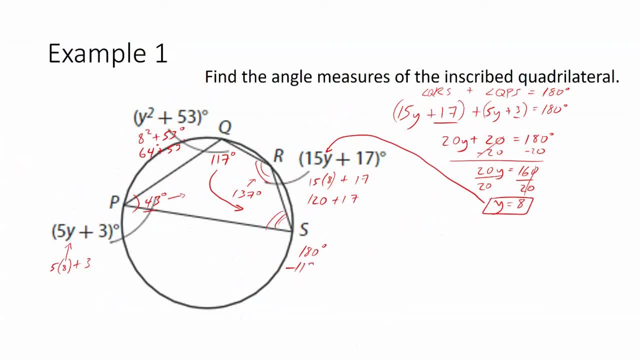 is again 180 degrees, minus the 117 that we got on the opposite side and that should get you- and don't forget to carry the one- 63 degrees. so there you go. so again knowing that theorem really does pay off in just solving and finding your angles. all right. example two. so here's another example: find the measures for the. 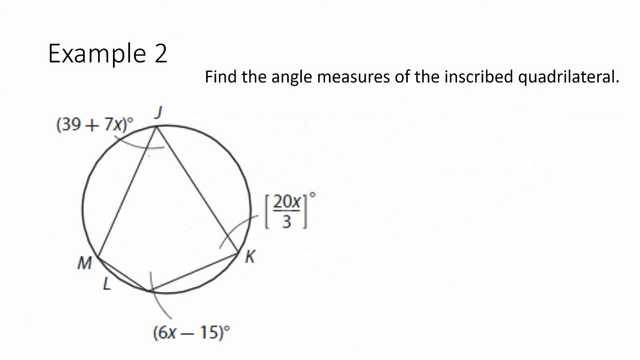 inscribed quadrilateral: um, looks like we're solving for x, right, because x is going to give it to you. and then again that нас觉得 it was. if we normally do this for x, let's say we add an x and then here you go. after that i'll write plus one over here. all my angles can be. 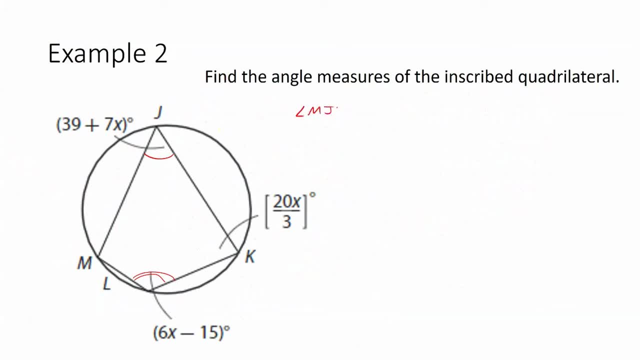 감 m jk plus m l k. here we go, angle mj k right, knock, knock, and i'll do it again. so here we go. angle m jk plus angle mlk. all right, should equal 180 degrees, right? we have on our property, so we have, i want to rewrite mlk. you should give us 180 degrees, so we have, i want to rewrite mlk, right? so nope, we're just going to write mj 2. it should equal 180 degrees. so that's all we have, all we have. so we're just going to do all of these and that should add up to 180 degrees, think is. 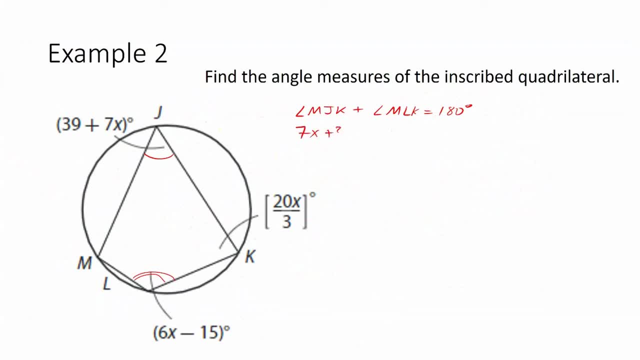 mjk, 7x plus 39 degrees right, plus angle mlk. all right, which is 6x minus 15 equals 180 degrees, and the rest is just algebra, right, combined like terms. so I'll combine the constant terms 39 minus that 15, you should get 24, and then the 7x. 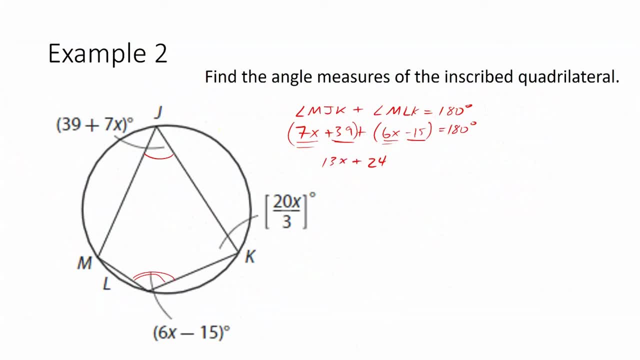 plus the 6x, 13x, and that should be equaling 180 degrees subtraction property. just don't forget: what you do to one side, do to the other right. so we got 13x equaling 156,. 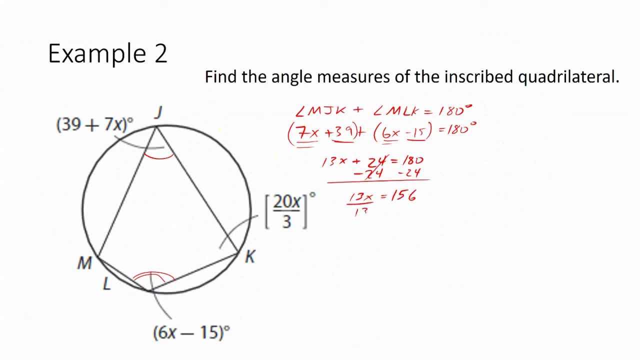 and then division. right, because how do you get rid of a multiplying 13,? multiply and again, what you do to one side, you do to the other, and you should get x equals 12, so again, that is not your answer. you are in geometry.